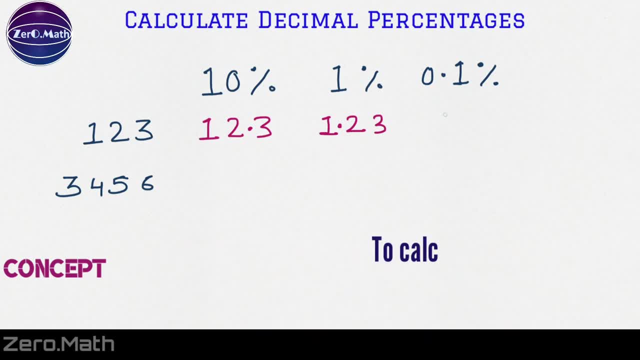 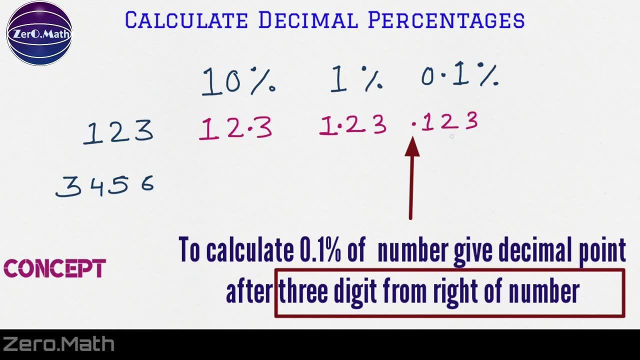 two digits from right hand side And 0.1% of 1,, 2, 3 would be 0.123.. Just give this decimal point 1,, 2, 3 places from right hand side. This is the concept you should fit in your head. Now let's. 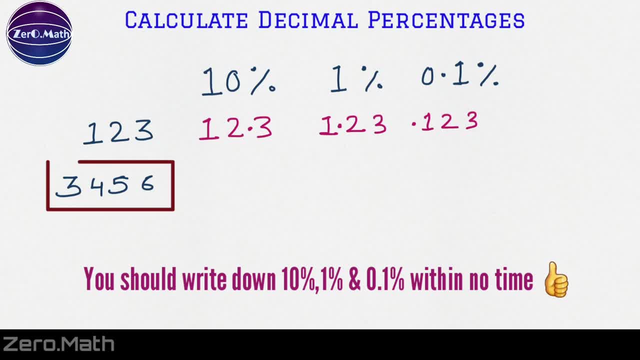 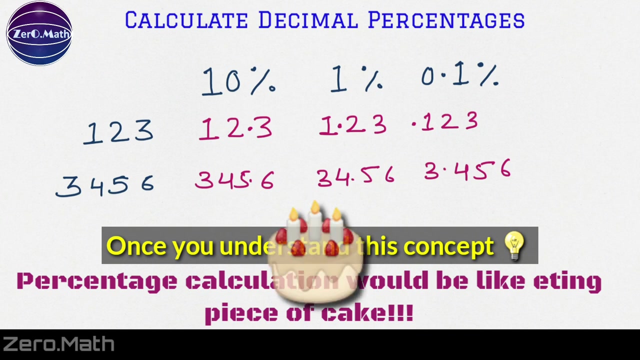 figure out 10%, 10% of 3, 4,, 5, 6.. So, without any second thought, you can write down the answer. The 10% of 3, 4, 5, 6 would be 3, 45.6.. 1% would be 3, 4.56.. Just give decimal point two digits from right hand side And 0.1% would be 3.456. If you are clear with the concept, then calculation of percentage for the decimal numbers. 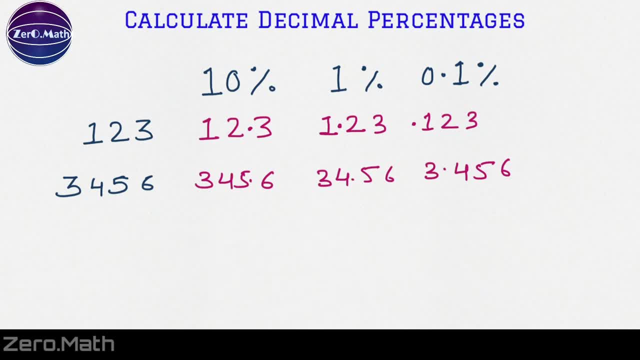 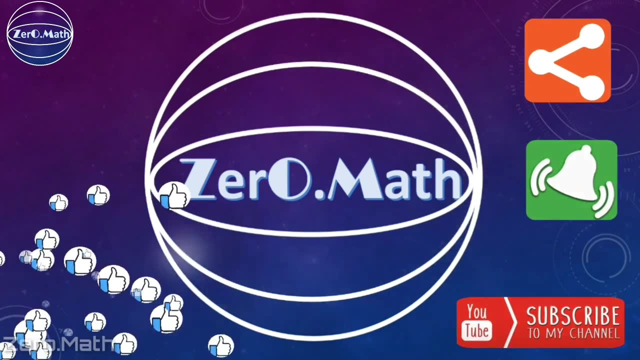 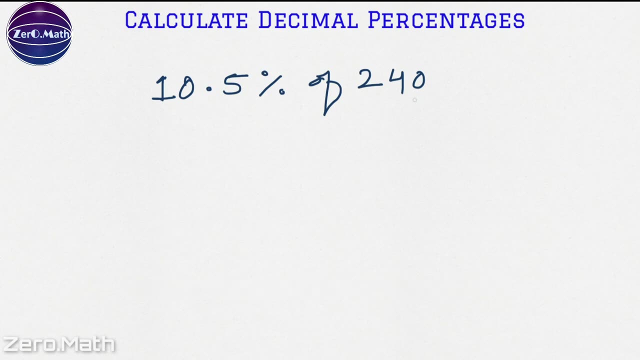 would be like eating a piece of cake for you. Let's start solving some decimal percentages problems. Let's begin with the simple sum. Let's calculate 10.5% of 240.. So what we are going to do? we are going to split this 10.5% as 10% plus 0.5%. 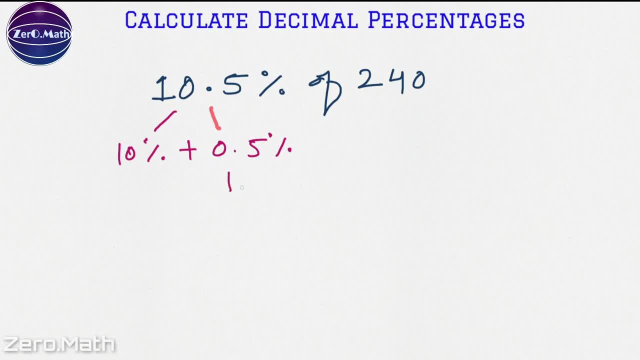 Now this 0.5% I can represent as 1% over 2.. Why I have converted this? because we know how to calculate the 10%, 1% and 0.1% Right? We know that concept. So let's calculate now 10% of 240. So it will be 24.0.. That is 24.. Just give this decimal point after one digit from right hand side, And what is 1% of 240?? 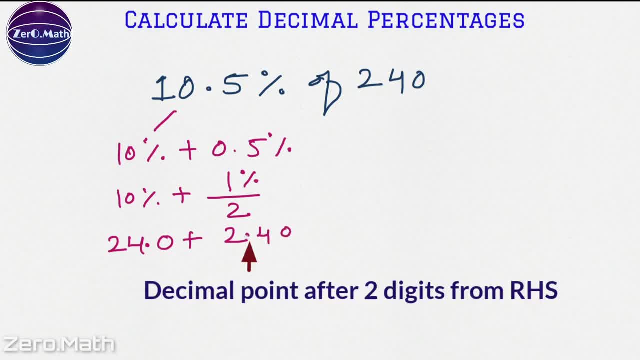 That will be 2.40.. Just give this decimal point, two digits from right hand side, divided by 2.. So our answer will be 24 plus 2.4 by 2.. That is going to be 1.2.. So the answer would be 25.2, which is 10.5% of 240.. Now you can see this 0.5%. I could have split it as 0.1%. 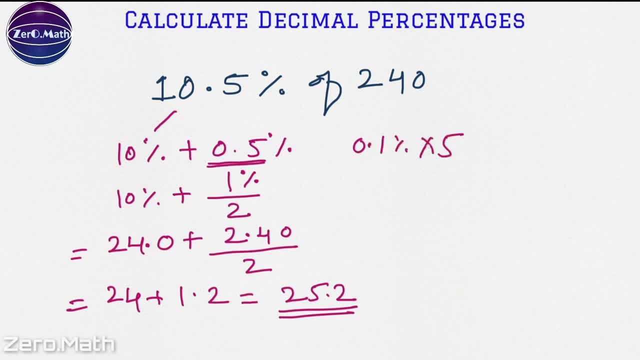 So again, using this also, I would have got the same answer. 0.1% of 240 will be 0.240.. Give the decimal point from three digits from right hand side into 5, which is equal to 1.2.. So you can see, using this as well, I would have got the same answer. 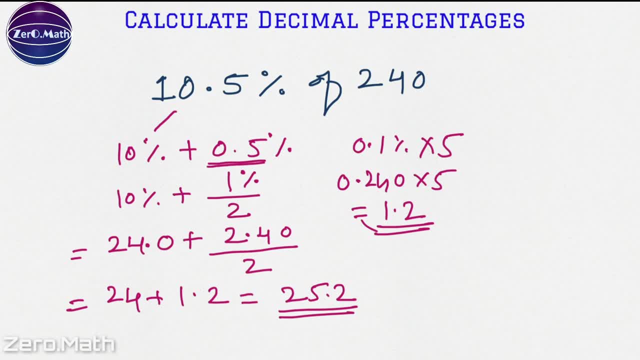 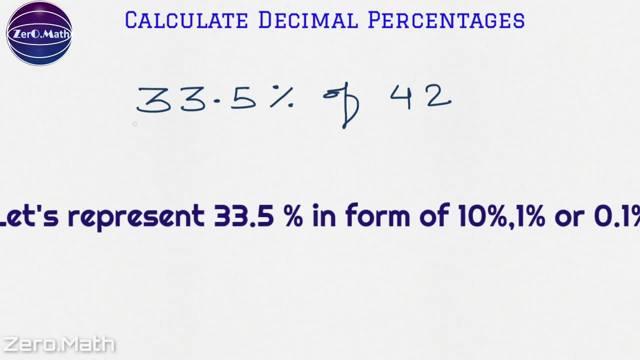 It's up to you which way you would like to solve it: 33.5% of 42.. So we will represent this 33.5 in terms of 10%, 1% or 0.1%. So 33.5, I can say it is 3 times 10%, which is equal to 30 plus 3 times 1%. So 3 times 1% is 3.. So 30 plus 3 is 33 plus half time 1%. 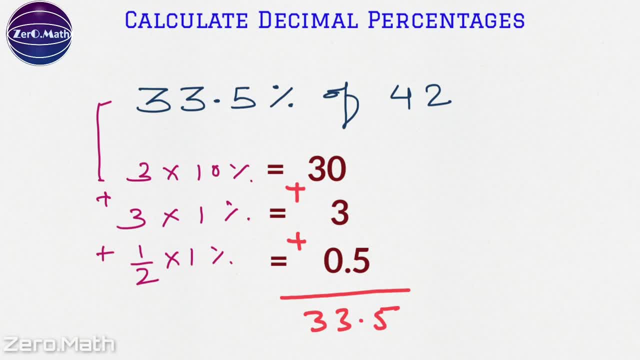 So, which is 0.5.. So it will be 33.5.. Now it will be 3 times. So what is 10% of 42? 10% of 42 would be 4.2.. Just give decimal point from one digit from right hand side. 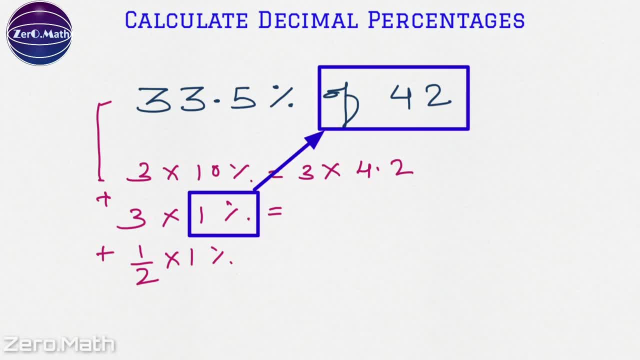 What is 1% of 42?? So it will be 3 times 0.42.. Right, Just give decimal places after 2 digits from right hand side. And what is 1% of 42?? It's again 0.42.. Let's add it up to get the answer. 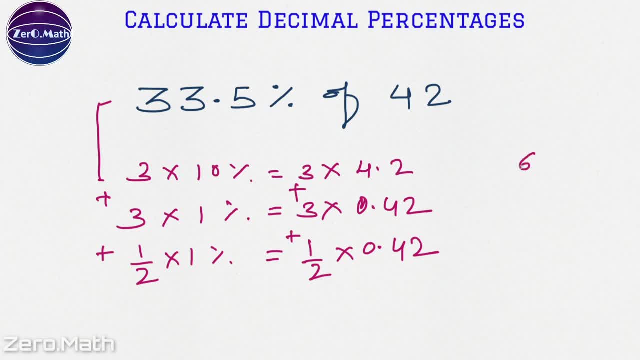 So what is 3 into 4.2?? So 3 into 2 is 6.. 3 into 4 is 12.. So it's 12.6.. Just give this decimal point after one digit from right. So what is 3 into 0.42?? So it will be again 1.26.. 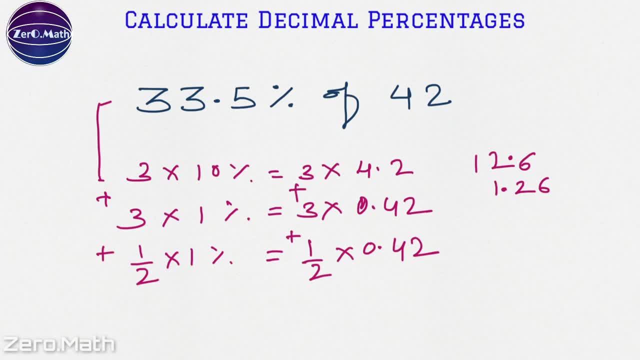 Just give decimal point after 2 digits from right hand side, And half of 0.42 is 0.21.. Let's sum it up So 6 plus 1 is 7.. 6 to 8 to 10 carry 1.. 2 plus 1 is 3 plus 1 is 4.. 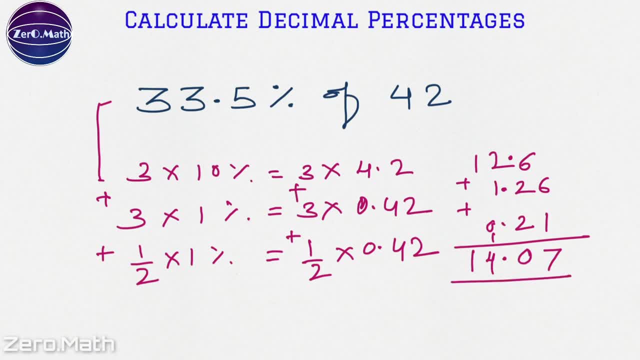 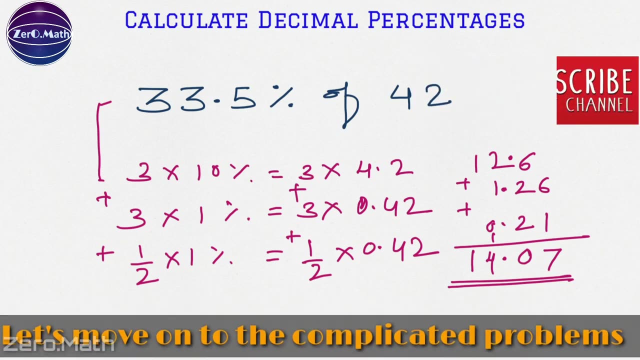 And this 1 as it is, I will give this decimal point. So 14.07 is the answer. So 14.07 is 33.5. And 35.5% of 42.. I hope you are enjoying this video. Let's move on to the complicated sums now. 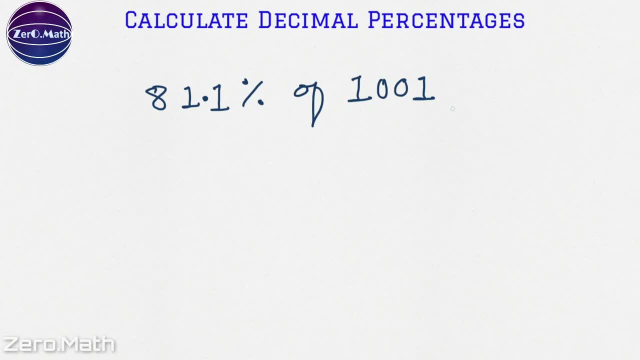 Let's quickly find what is 81.1% of 1001.. So let's split this 81.1%, So it can be split as 8 into 10%, which is equal to 80% plus 1%. It will be 81% plus 0.1%, So it will be 81.1%. 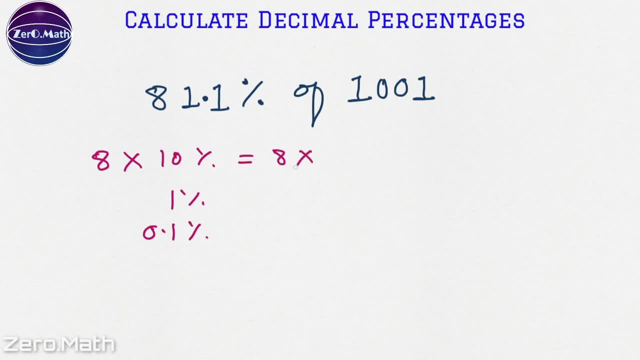 So it will be 81.1%. So it will be 81.1%, It will be 8 into what is 10% of 1001. that is going to be 100.1.. Just give this decimal point after one digit from right hand side. 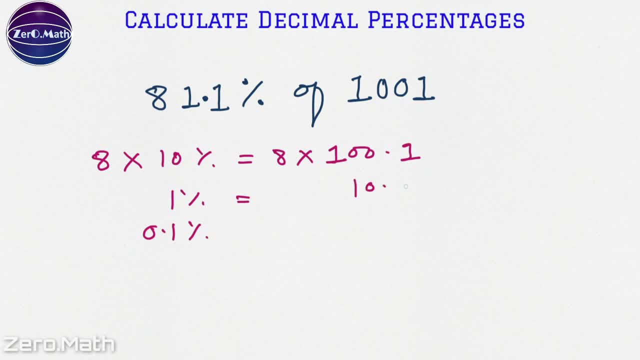 What is 1%, that is going to be 10.01, and what is 0.1%, that is going to be 1.001.. Let's add it up. Actually, this step 8 into 100.1. you can do it in mind as well. 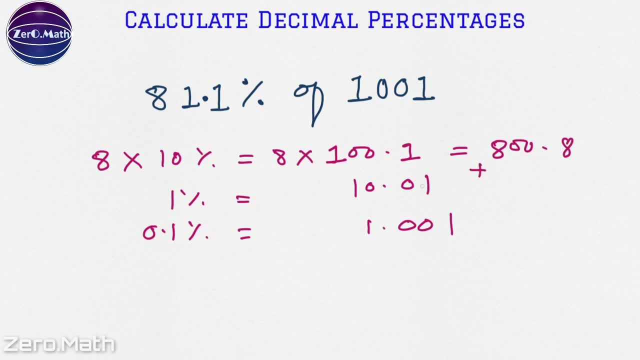 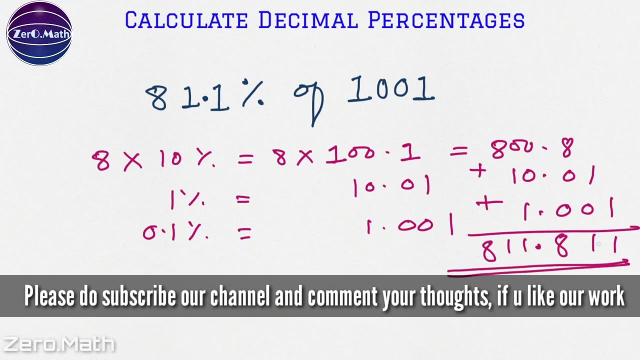 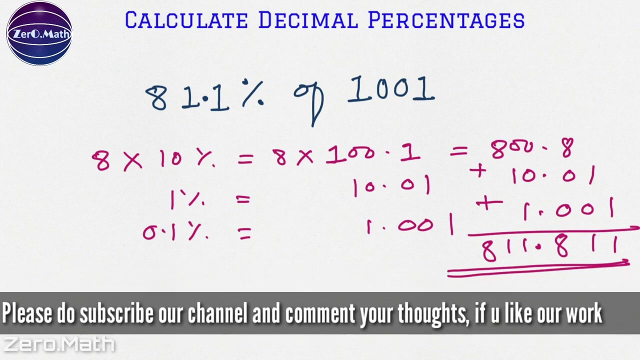 So it is going to be 800.8 plus 10.01 plus 1.001.. If you add it up, you will get 118.. This point as it is 118.. So 811.811 is our answer. So 81.1% of 1001 is 811.811. 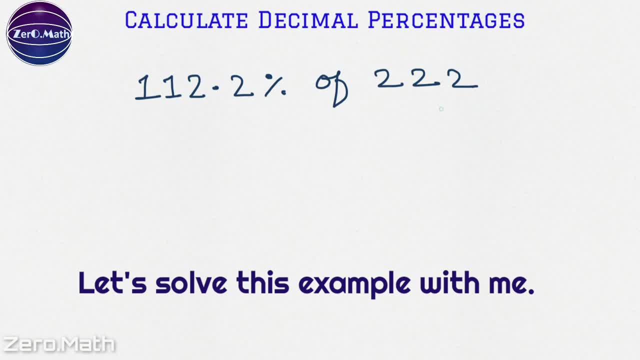 Let's solve this final example. Let's try to find out Answer with me. as a practice sum, Let's figure out what is 112.2% of 222.. So 112.2 can be splitted as 100% plus 10%. 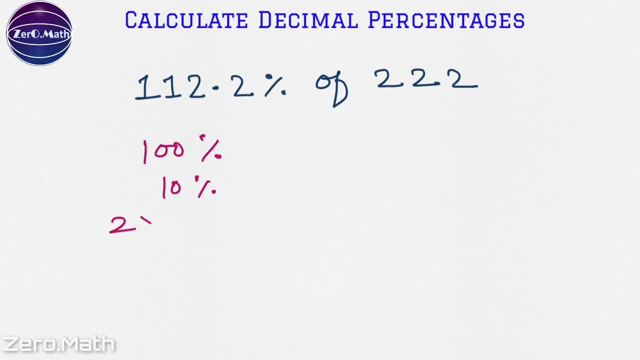 So it will be 110 plus 2 into 1%. So it will be 112 plus 2 into 0.1%, So it will be 0.2.. So we will get 112.2.. So what is 100%?